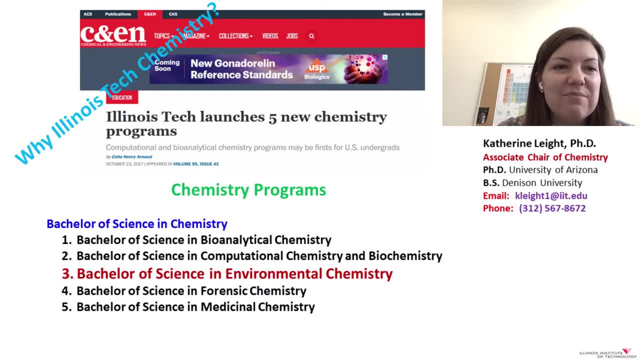 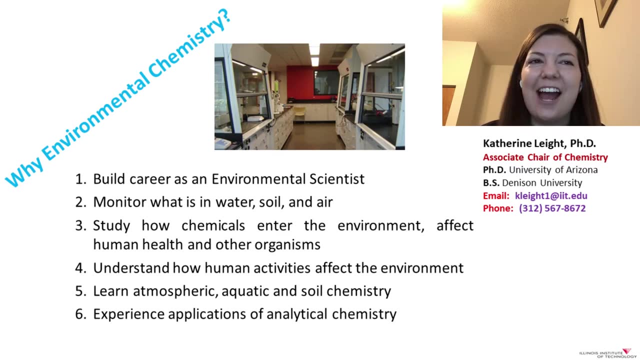 from. Most of them are unique in the Chicagoland area. You'll be very happy to know that all of these programs are accredited by the American Chemical Society. Our environmental chemistry program will help you build your career as an environmental scientist in environmental protection agencies. As an environmental chemist, you will advise on 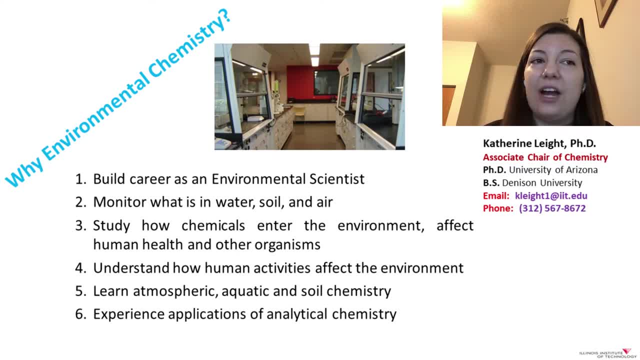 the movement and outcome of contaminants in groundwater and soil, assess long-term risks to human and ecological health, apply for environmental permits to undertake corrective strategies, classify contaminated soils as hazardous waste and manage their disposal and supervise on-site remediation. Last but not least, our environmental chemistry is an interdisciplinary science that covers 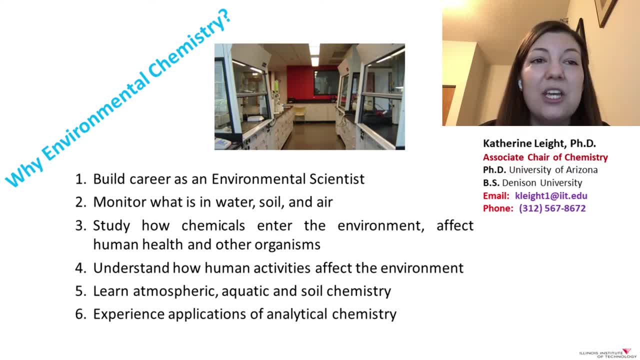 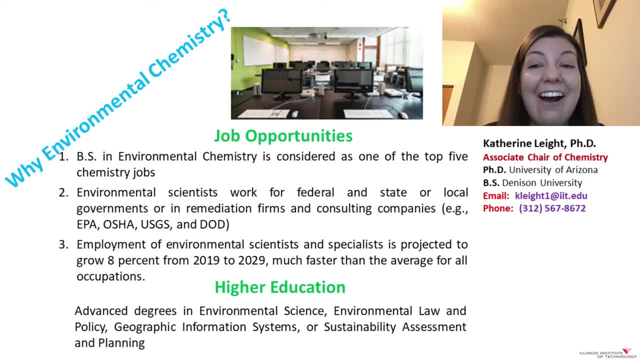 atmospheric, aquatic and soil chemistry, which are all heavily related to analytical chemistry. Obviously, you want to know your future. after getting a bachelor's degree in environmental chemistry from Illinois Tech, You have two clear paths, The first being that you can declare yourself as a potential employee. 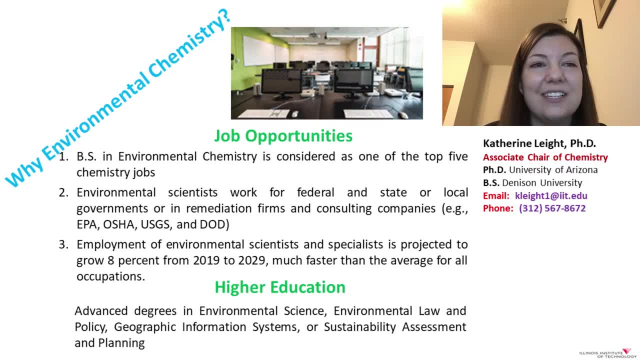 Job opportunities in this field are very good for many reasons, The first being that a bachelor's of science in environmental chemistry is considered one of the top five chemistry jobs. Second, great opportunities to work as an environmental scientist in the EPA, OSHA. 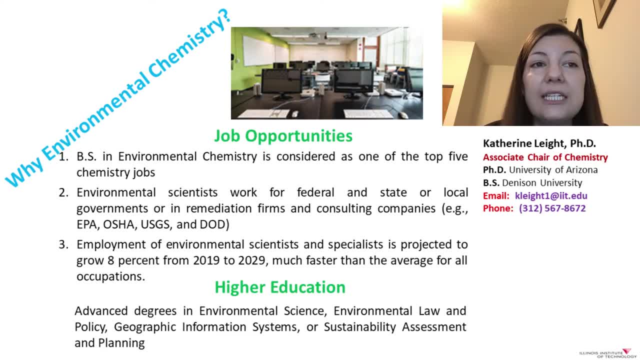 USGS and DOD labs or in a remediation firm and consulting companies. Finally, I found this quite exciting: employment of environmental scientists in specialties is projected to grow 8% from 2019 to 2021.. Thank you, 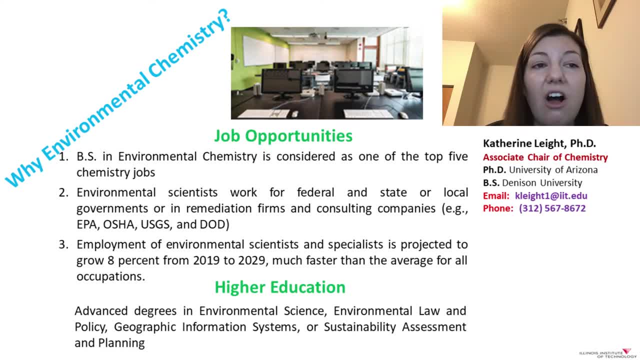 And the second pathway being that obviously deals with higher education. This pathway is always going to be open to you. You can specialize in environmental science, environmental law and policy, geographic information systems or sustainability assessment and planning. I personally favor the path that involves study, study, study until you are satisfied. 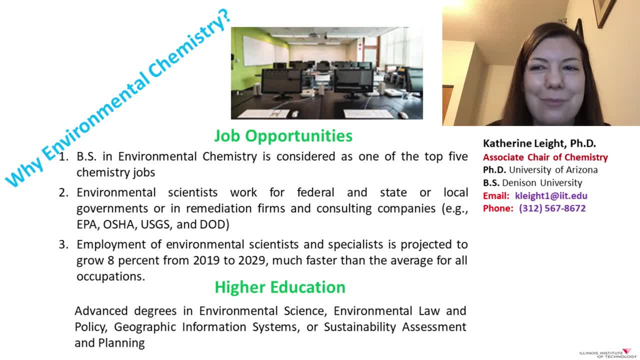 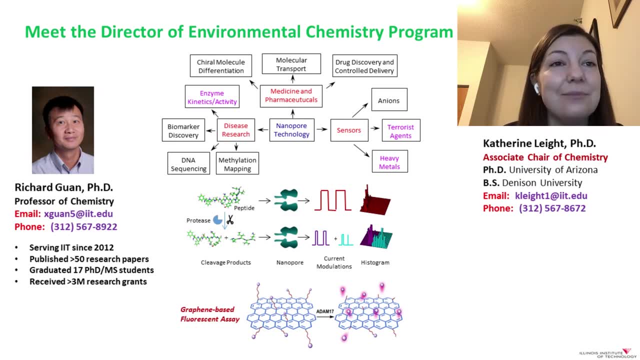 This is just a brief introduction of our environmental chemistry program. I strongly recommend that you immediately contact Professor Richard Guan, who is the director of our environmental chemistry program. He can set you up with a virtual meeting with you and possibly with your parents, to address. 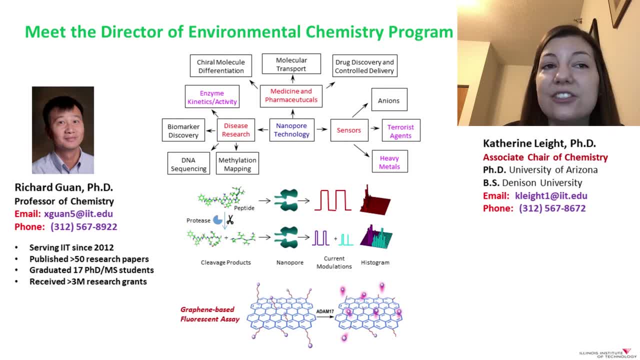 all of your questions involving the curriculum, opportunities for scholarships and research prospects during your undergraduate studies at Illinois Tech. For more information, please visit our website. the US Department of Science and Technology The University of Illinois is the home of the Illinois Institute for Environmental Science. 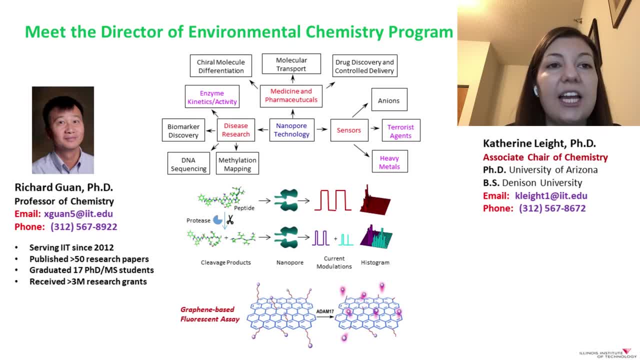 Undergraduate research is an integral part of our education at Illinois Tech. No matter which program you choose, you will have plenty of opportunities to perform cutting-edge research in a number of areas during your junior and senior years. For example, Professor Guan's research. 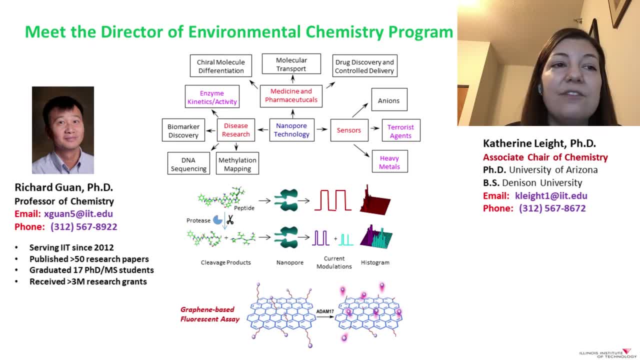 is centered on developing nanopore technology for various applications. It starts with synthesis of nanoscale-sized pores and involves a variety of analytical techniques to characterize these nanopores. You can work side-by-side with graduate students to create new materials capable of detection of environmental contaminants and biomarkers with much better sensitivities and 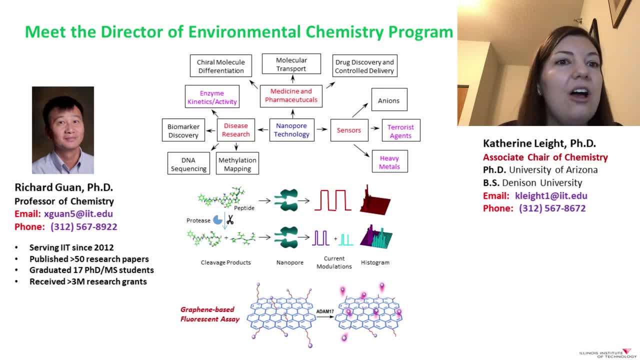 selectivities than those that are currently available. I am sure you will find an exciting research area for you to explore. Thank you for your attention. If you desire, you can also engage in a wide variety of clubs and activities that suit your interests. Some of the things I have been involved in with the students on campus is the Chemistry 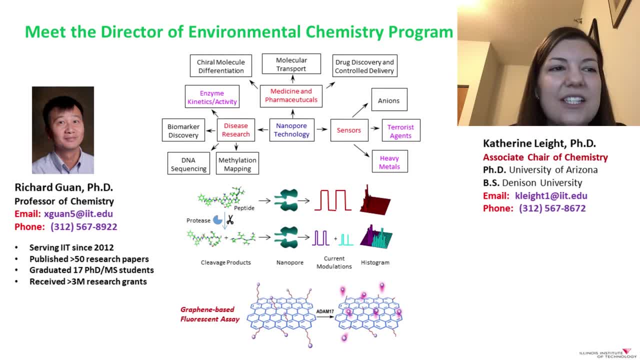 Club, who hosts social events, study sessions as well as fun chemistry demonstrations. Finally, I would like to emphasize that the passion of our department is to cultivate a student-first culture by engaging our students both in and out of the classroom. We strongly believe that our